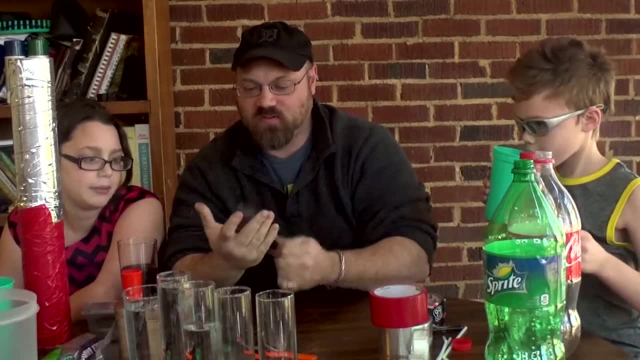 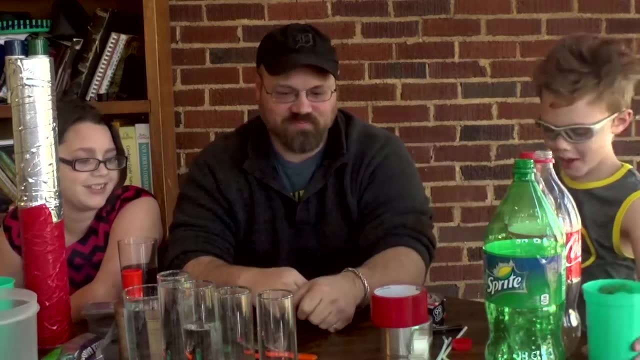 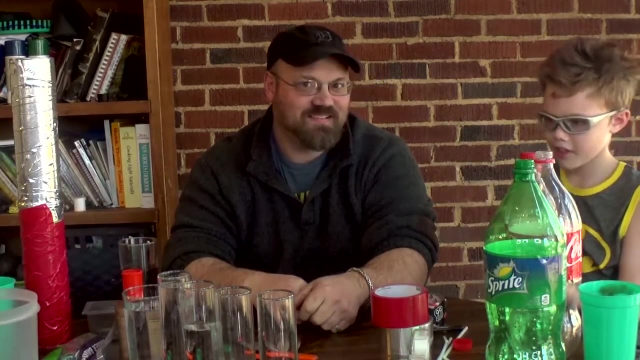 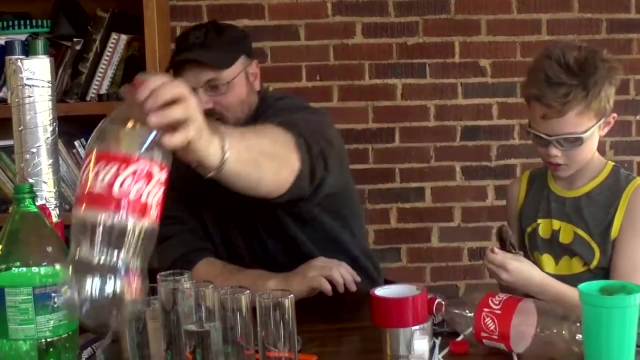 Ah, I'm losing my grip. Maybe you can tape it. You probably can tape it If you had like You try. That's your hand, Does it work? Let me see that clear tape. Maybe you can go like this. 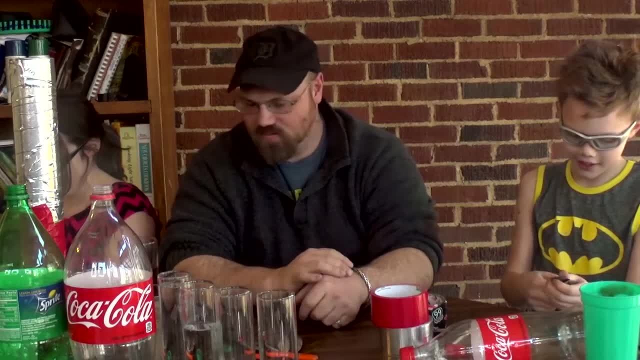 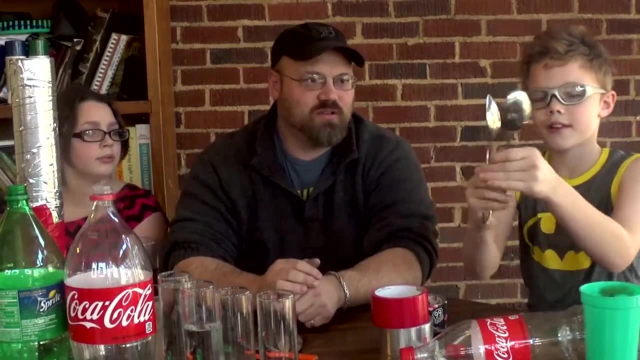 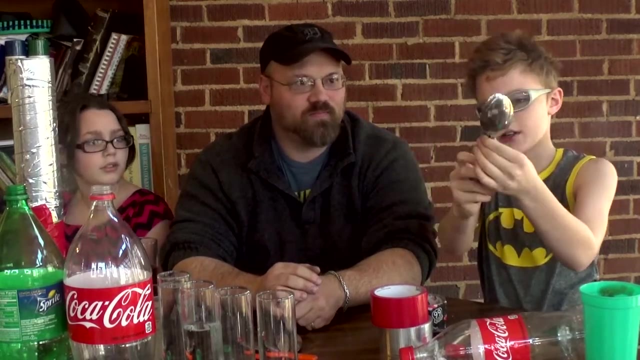 Well, yeah, you can do it that way too. That's another way to do it. So, Gideon, just found another way that you can do this, But this one that way, and the other one that way, and this one overlapping the other spoon. 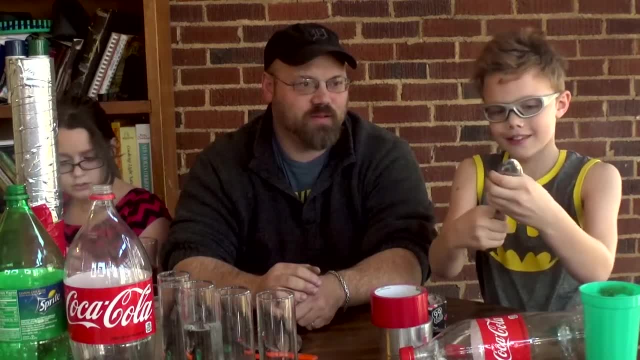 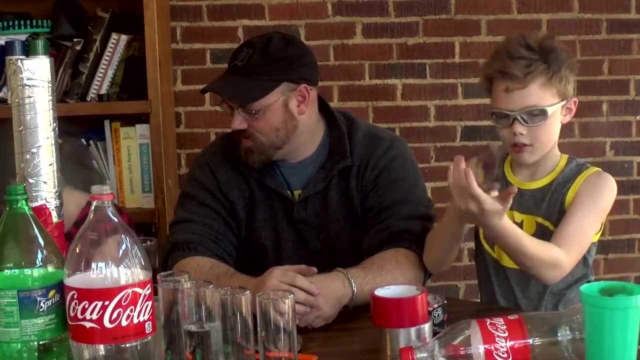 And then put your finger in between them, right, Instead of back to back, And then you whack it. Cool, I think that one works better. And will you tape them? Yeah, I think that one works better. Maybe you could tape them but put like a rolled up piece of something in there. 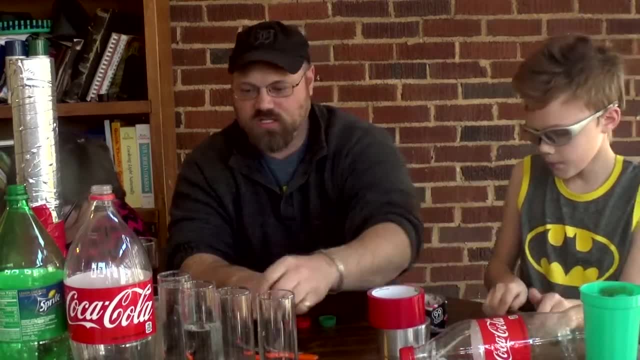 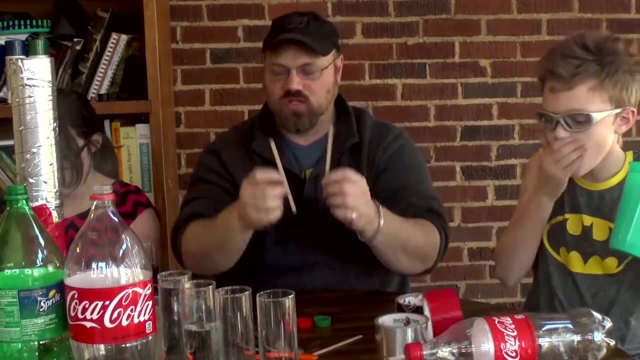 Another kind of clapper that you can make. that's pretty easy. Can I see that? Do you want me to do that tape for a minute? Etta, If you can find a couple old sticks, Actually, yeah, I'll use this tape. 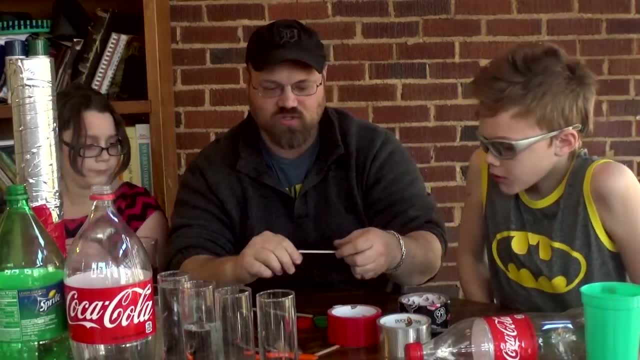 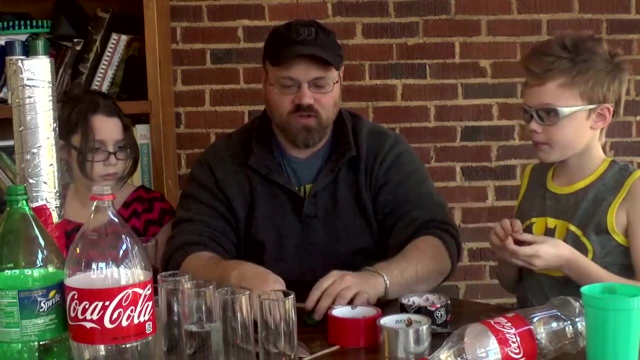 If you can find a couple little toothpicks or popsicle sticks or something like that around the house- I have a couple of craft sticks here- And if you can get a couple bottle caps, you can take a little piece of tape and you tear it off. 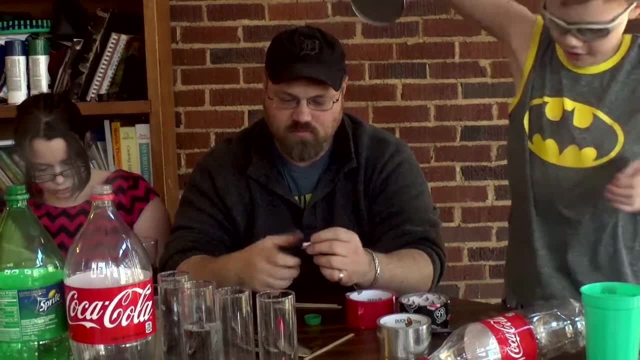 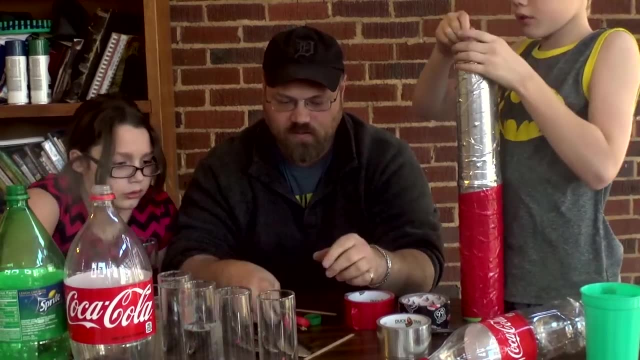 Can I do a trick or something? Yep, And you just wad it up like that. You wad it up on the end and put one of your bottle caps on there, And on the other one you do the same thing. What are you doing? 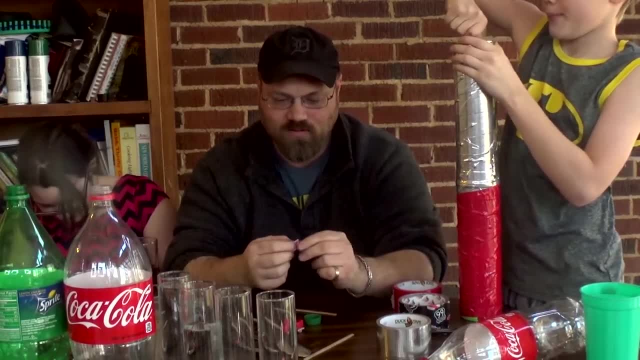 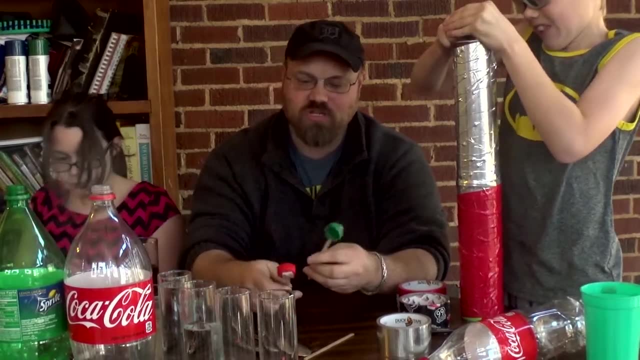 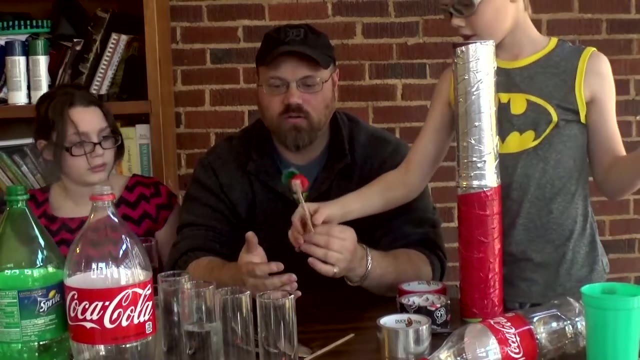 I have no idea. Okay, well, don't do that right now, And you put a piece of tape on the other end with another bottle cap, And then the bottle caps can make a little clacker too. It's not quite as loud. 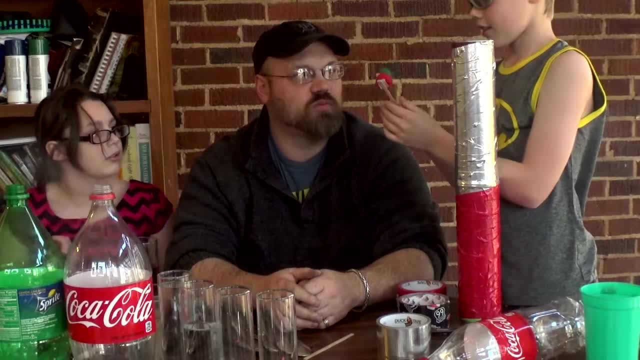 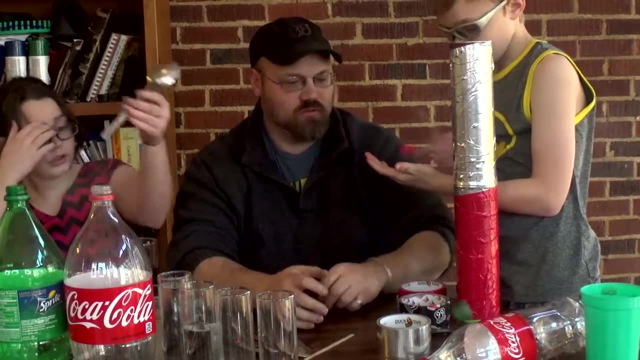 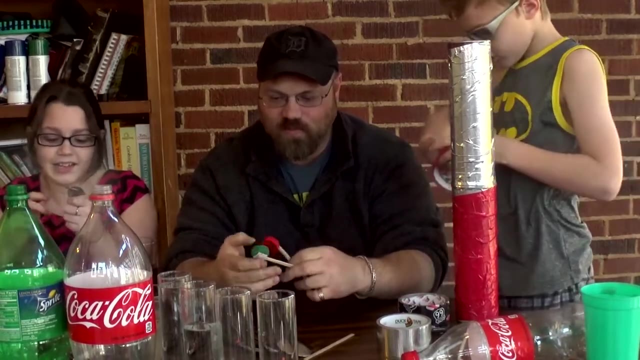 As the as the spoons, but it still works pretty good. Yeah, Can I try again? I don't think the spoon tape method worked. Okay, so we learned that. Or you could go like this: You could take this one.